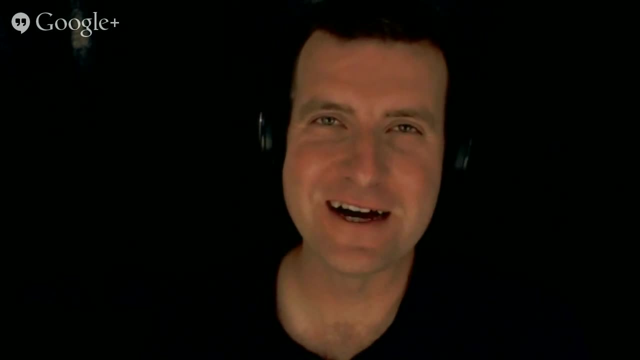 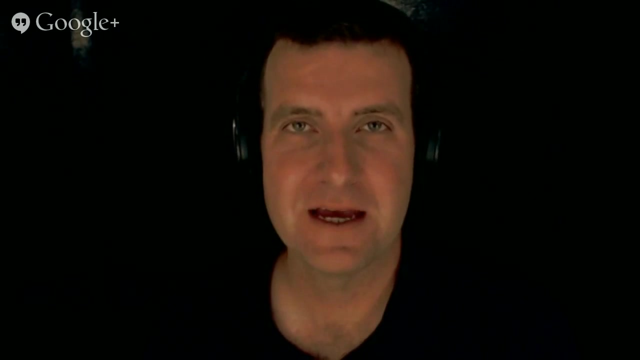 Hi again everyone. Chris Tisdale here again. In this presentation I am going to continue my series of videos on complex numbers. Now, in particular, I am going to show you how to solve a quadratic equation that has complex numbers as coefficients. So we will work through. 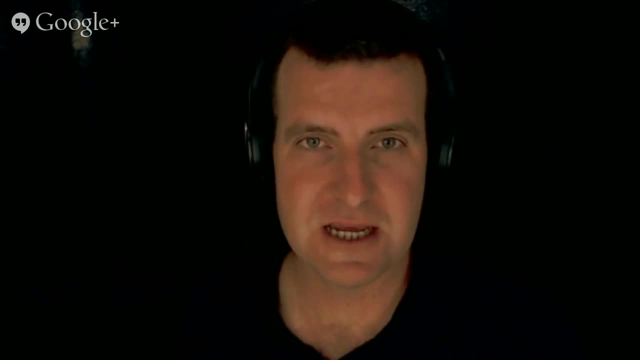 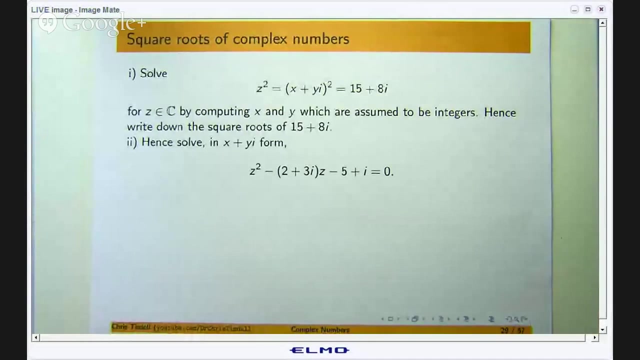 an example, and let me share my screen with you so we can get down to business. Okay so, square roots of complex numbers and quadratic equations that have complex numbers as coefficients. Okay, so it is a two part problem. We are going to solve the following. 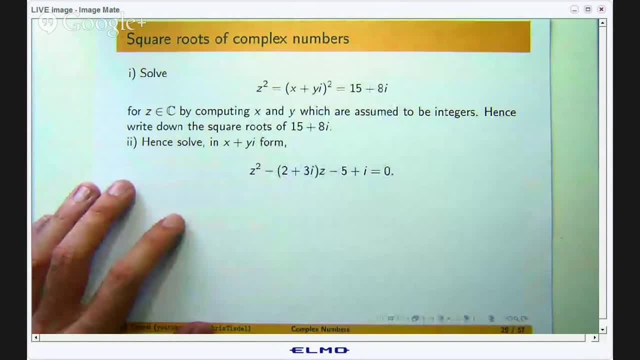 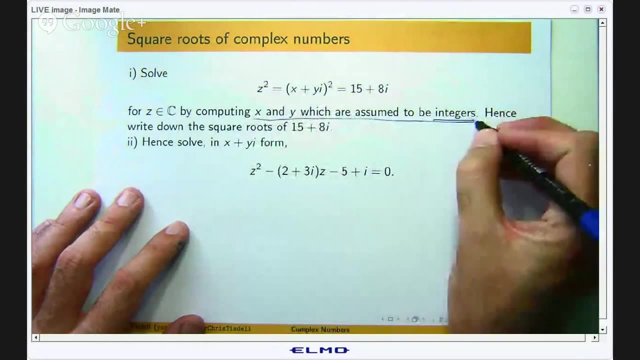 problem first, and then we will use that information in the second part. Okay, so we want to solve this. z squared equals 15 plus 8i. by computing the real and imaginary parts of z, We have z which are assumed to be integers or whole numbers. Now, this simplifies some of 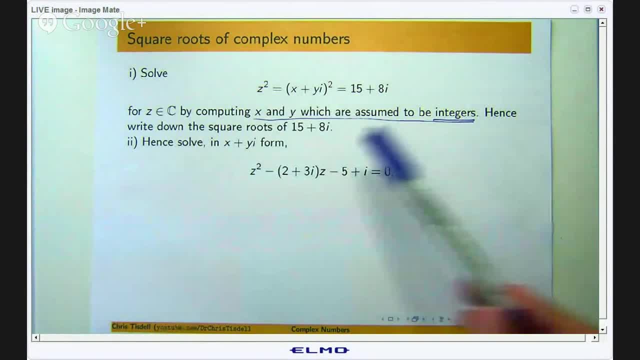 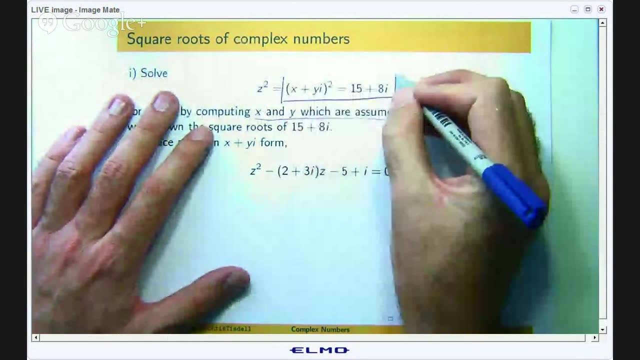 the calculations, Okay, and hence write down the square roots of 15 plus 8i, and we will use that in solving this, where we just apply the quadratic formula. Okay. so let us forget about the z and let us compute x and y. Once we know x and y, we have z. 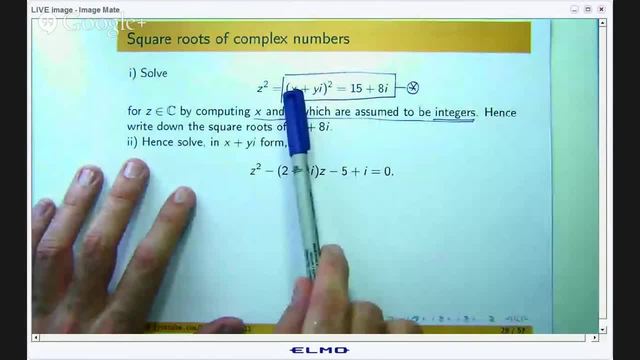 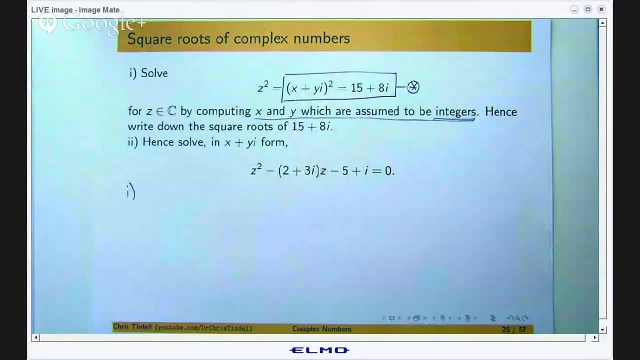 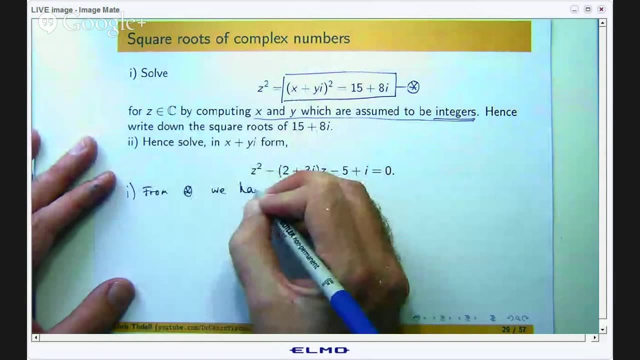 So how do we do it? Well, for part one, what we are going to do is expand this bracket and then equate the real and the imaginary parts. Okay, so let us expand the brackets. So when I expand this, I am going to get x squared and I am going to get yi all squared. 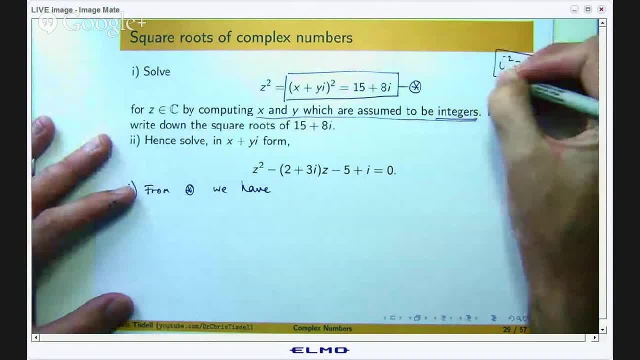 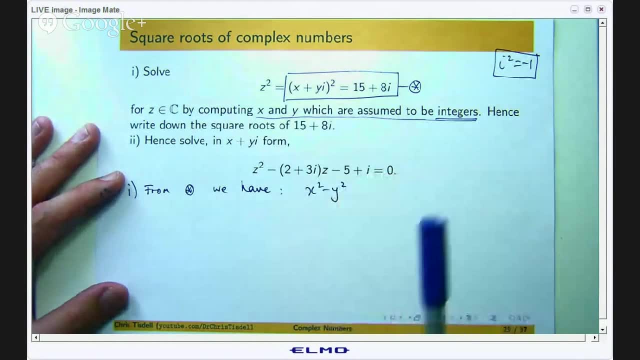 Now remember: i squared equals negative 1.. So I am going to get x squared minus y squared square. they are going to be the real parts and you are going to get 2 times that, times that, 2 x y i. So the imaginary part would be 2 x y and that has got to be equal to 15. 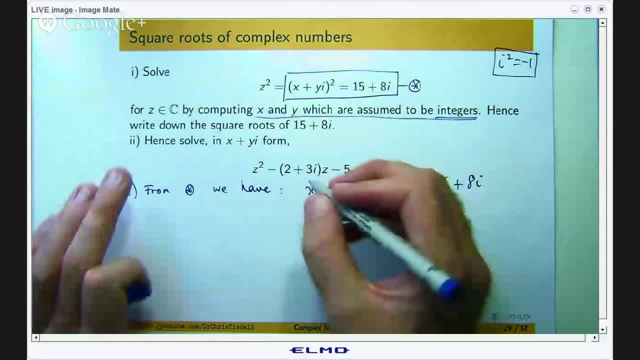 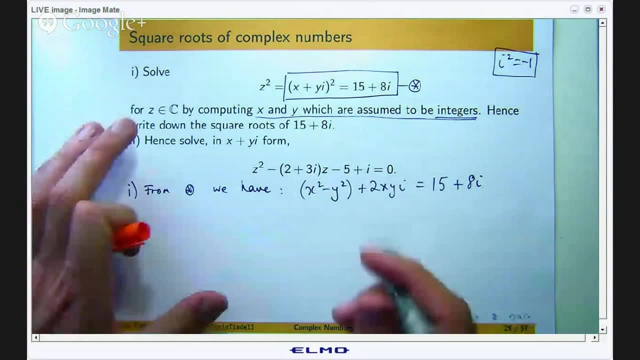 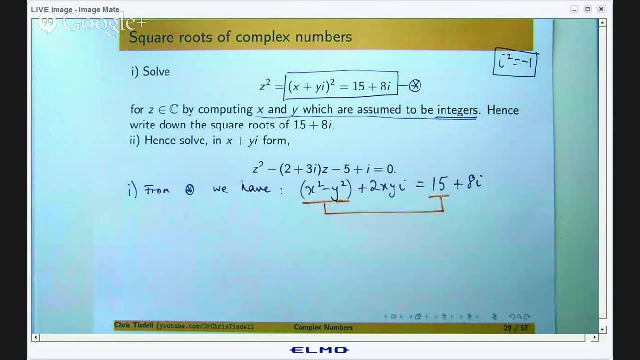 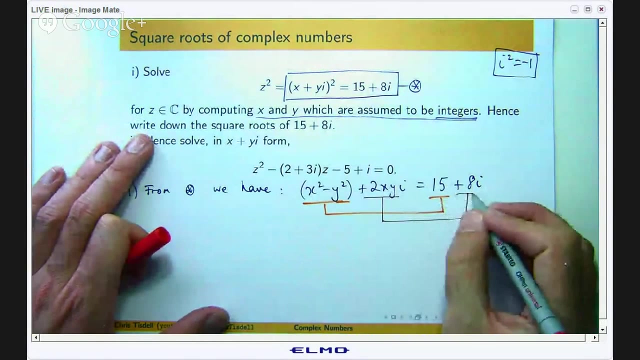 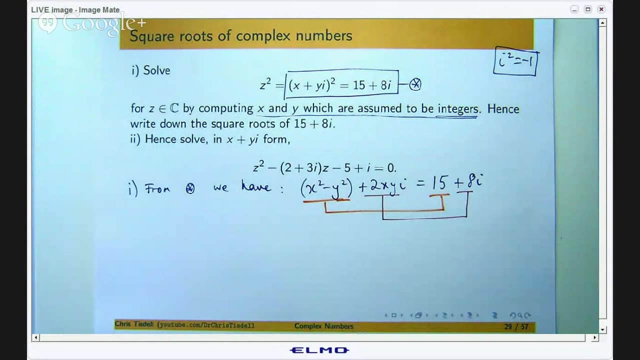 plus 8 i. So two complex numbers are equal if, and only if, their real parts are equal, so that and that are the same, and their imaginary parts are equal, So that 2 x y has to equal 8 or positive 8 over there. So if we equate those, we set them equal, we will get two equations. 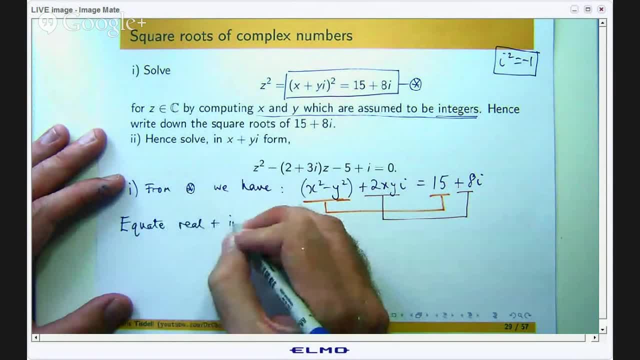 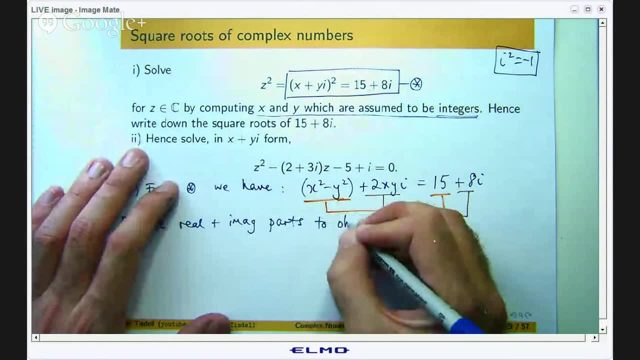 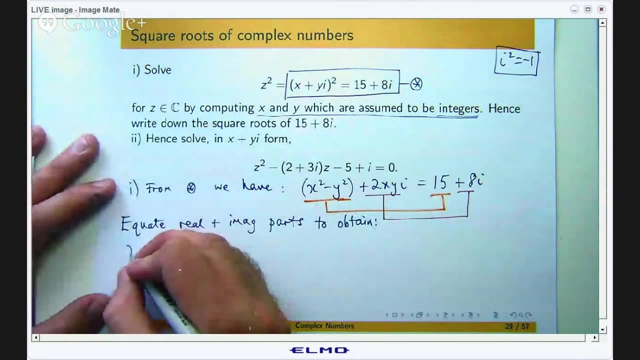 So let us equate the real and imaginary parts. So that is the real and the imaginary parts. So that is the real and the imaginary parts. Okay, so we are going to get x squared minus y squared equals 15.. That is one equation. 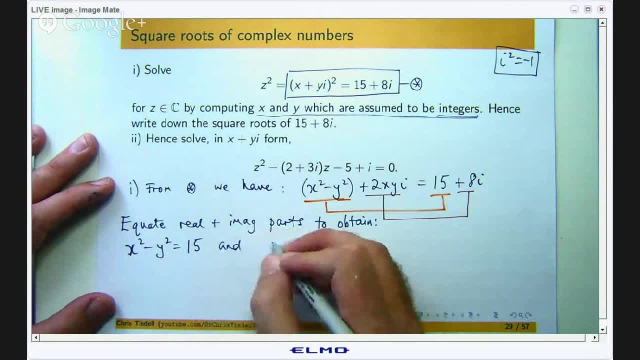 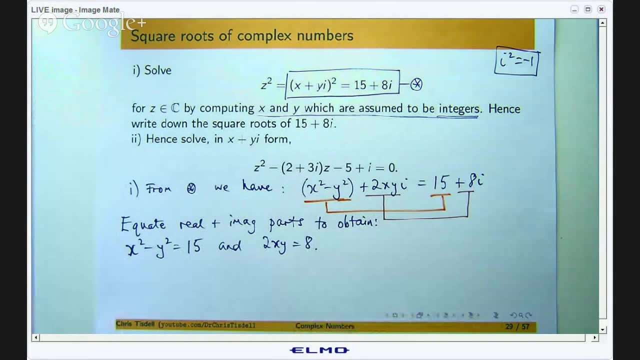 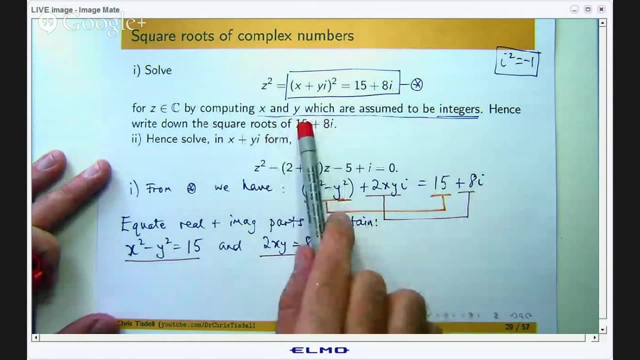 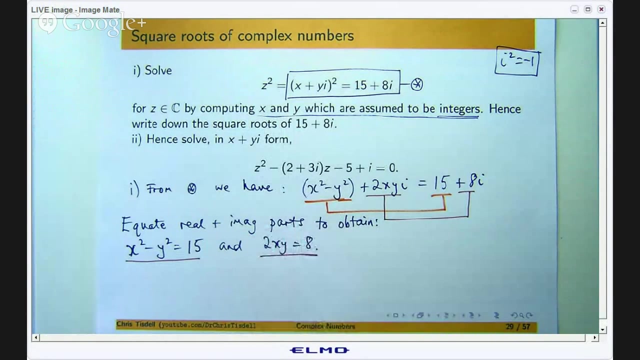 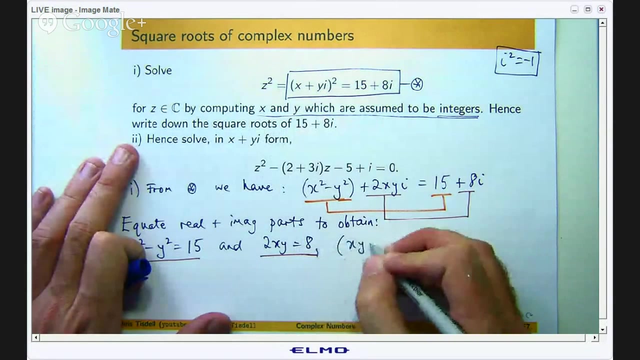 and 2, x, y equals 8.. okay, so how do we solve these? Well, the nice thing Now is that, because we know, given the knowledge that x and y are both integers, are both whole numbers, we can actually start with this and say: take the 2 to the other side. 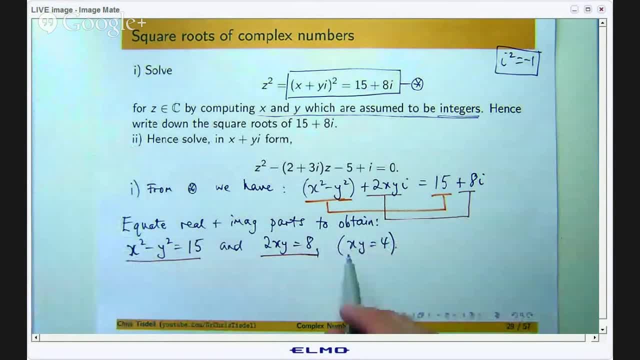 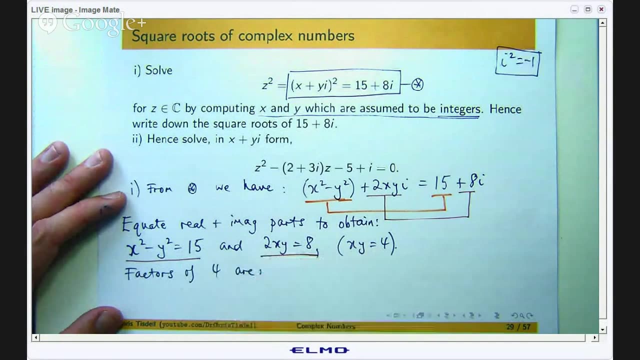 And then I can come up with potential values for x and y just by looking at the factors of 4.. Factors of 4 are the following: let us say 2 and 2, negative 2 and negative 2, 4 and. 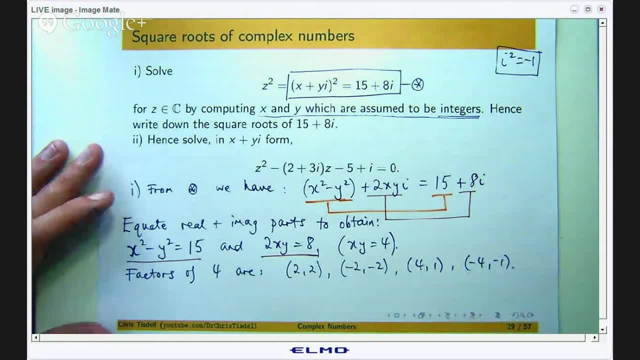 1, and negative 4 and negative 1.. Now we cannot have all of those, but we can rule some of them out. Let us put x equals 2.. y equals 2 in there, you do not get 15.. Same with x equals negative 2 and y equals negative 2, you put those in there, you do. 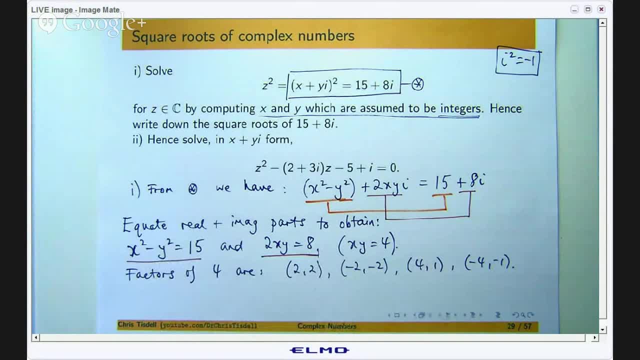 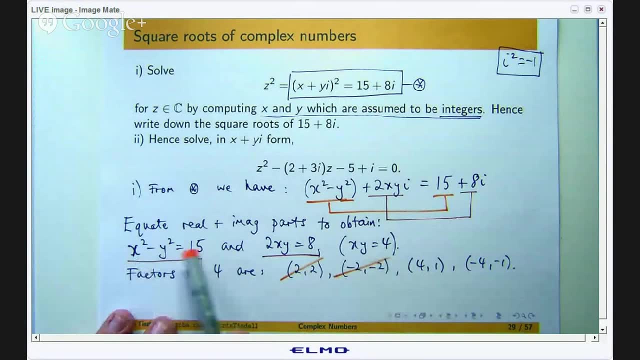 not get 15.. So those two can actually be scratched out because they do not satisfy that equation. What about these two? Well, if x equals 4 and y equals 1, you will get 15 and same with negative, 4 and negative. 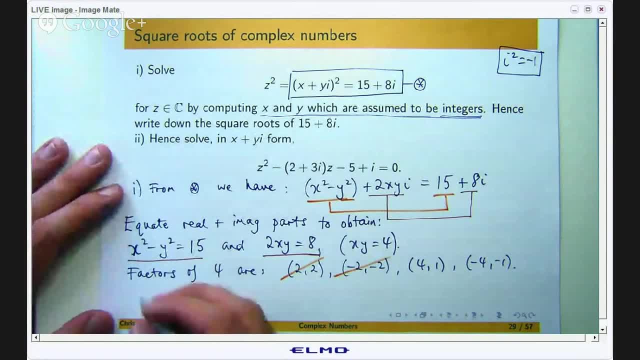 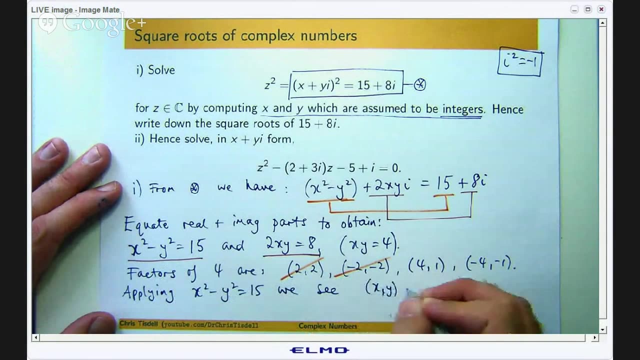 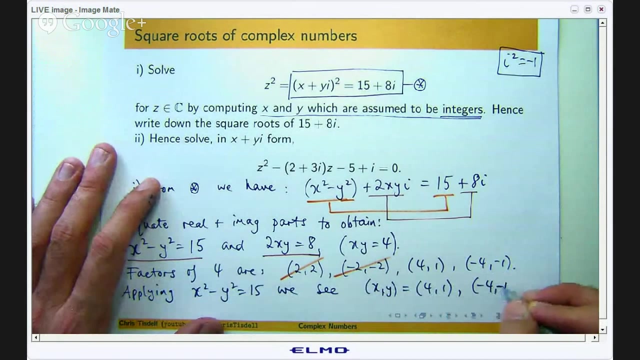 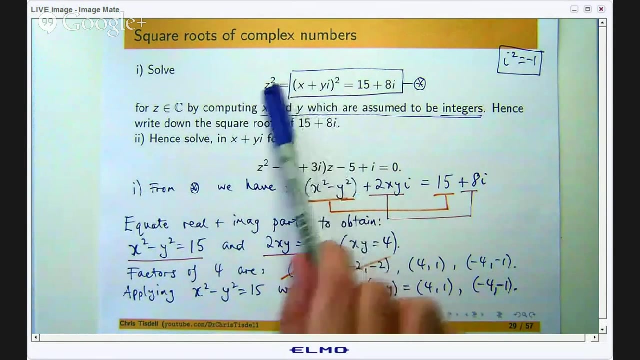 1.. So if we apply x squared minus y squared equals 15, we see that x and y is 4 and 1, or negative 4 and negative 1.. Okay, so there is going to be two complex numbers that satisfy this. 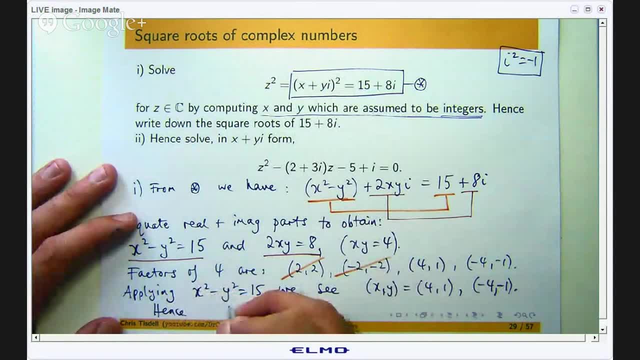 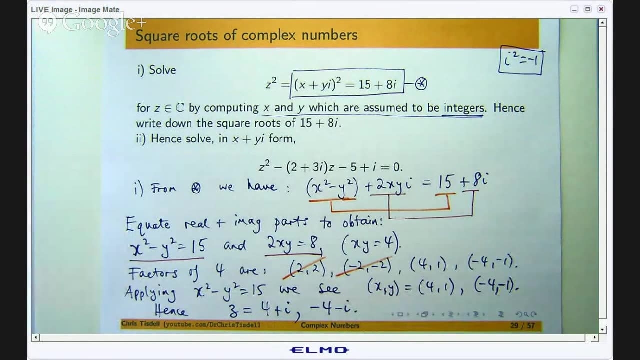 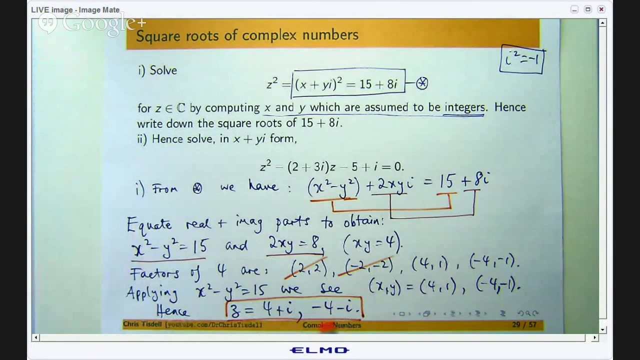 Okay, Okay, Okay, And it is going to be 4 plus 1i or just 4 plus i, and negative 4 minus 1i or negative 4 minus i. Alright, so these, then, are the roots of 15 plus 8i. 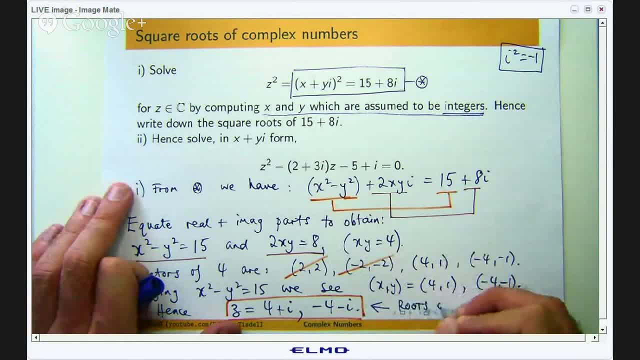 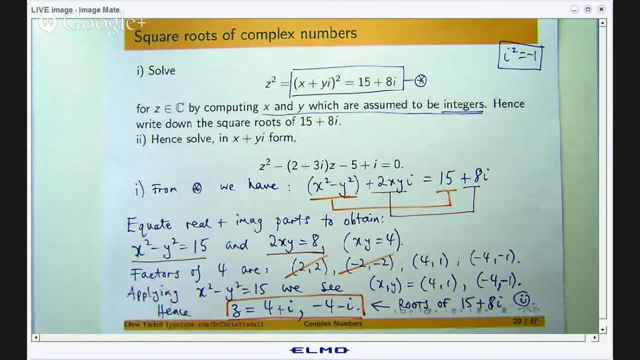 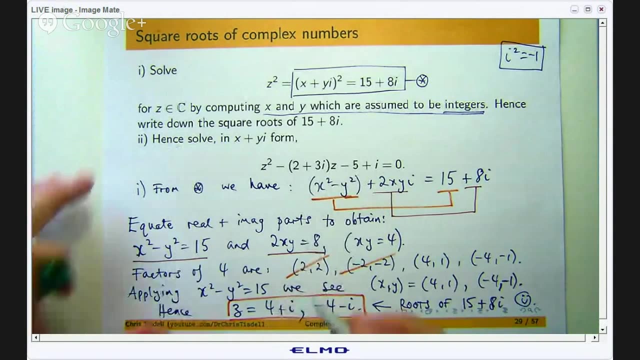 Okay, Okay, Okay, Okay. So that is the first part done, So let us go and see if we can solve the second part Now. the second part is just looking at a quadratic equation, which you have seen quadratic equations at high school. 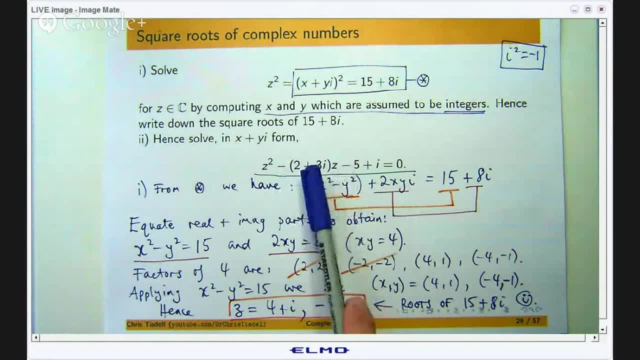 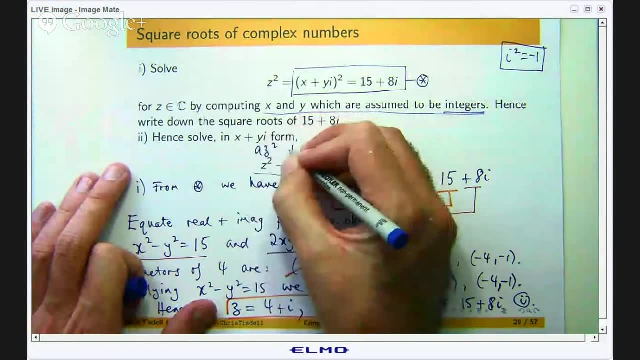 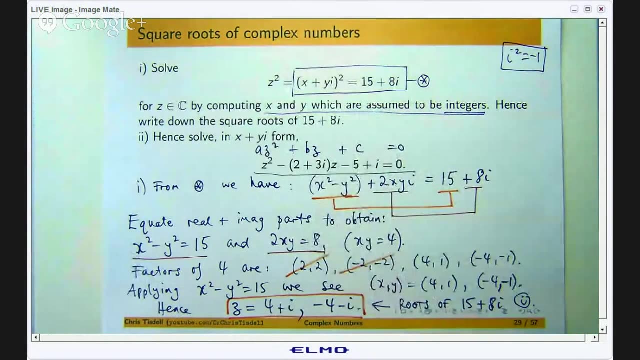 But this one has a twist. You are using, you have got- coefficients that are complex numbers, Okay. So we have still got it in the form a. say z squared plus bz plus c equals 0. But b and c are both complex numbers. here a is just 1.. 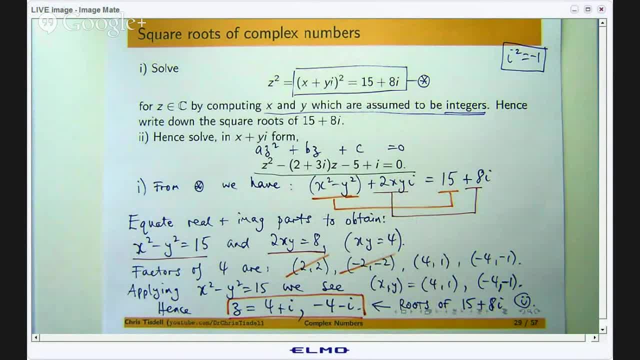 What we are going to do is apply the quadratic formula to solve this, and actually the square root sign that we are going to get is going to be the square root of 15 plus 8i. So we are going to use part 1 to solve part 2.. 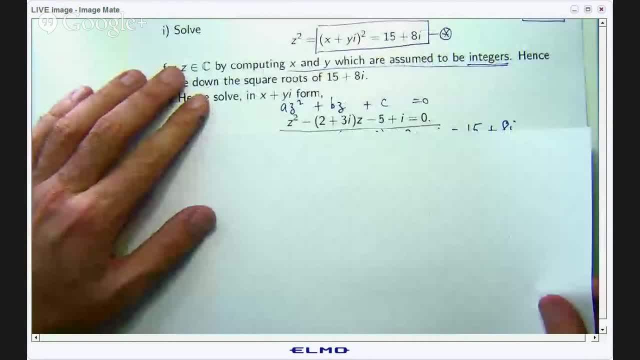 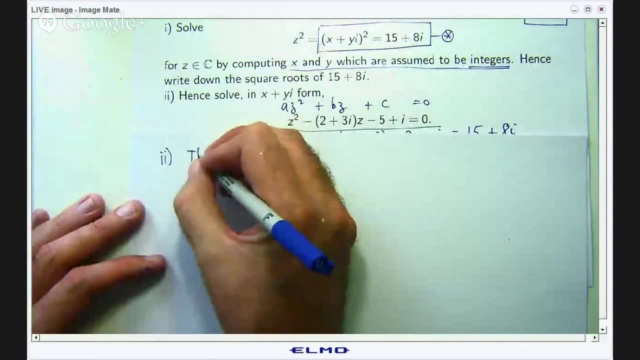 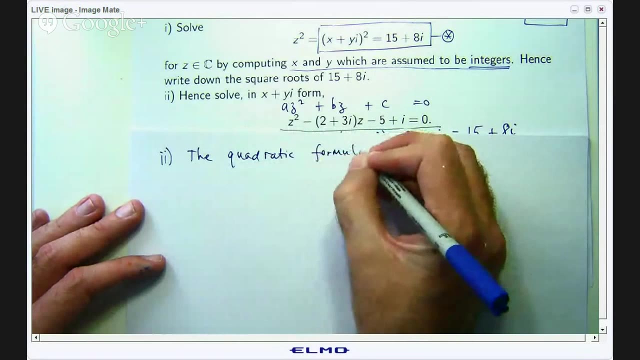 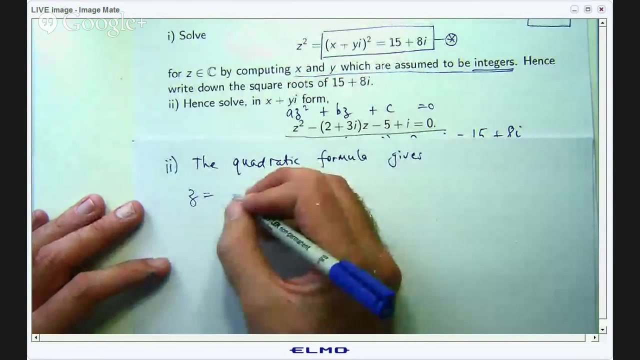 So let me show you how that works. Okay, So we are going to apply the quadratic formula that we all know. Okay, We know that z is going to be negative, b plus or minus the following square root: all over 25.. Okay, 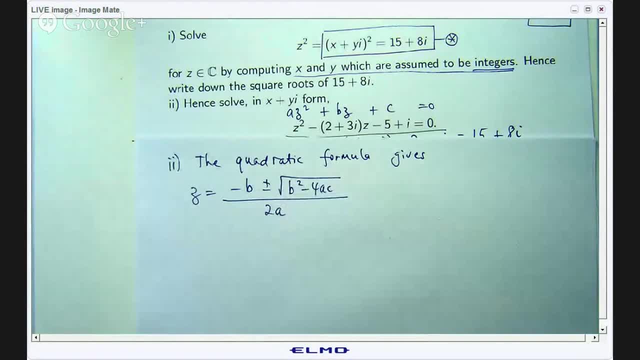 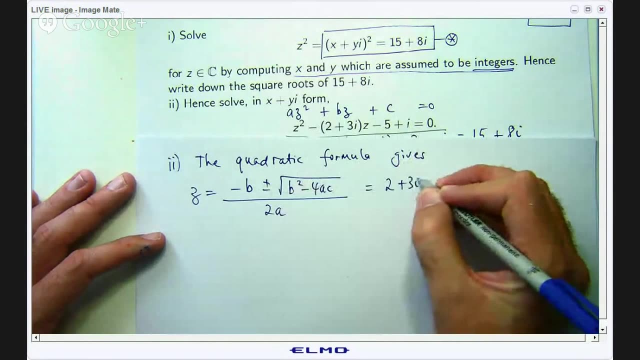 Okay, Okay. So b in this case would be negative all of 2 plus 3i, A would be 1 and c would be negative 5 plus i. So if you put those in here, you will get the following: So the negative will cancel out. 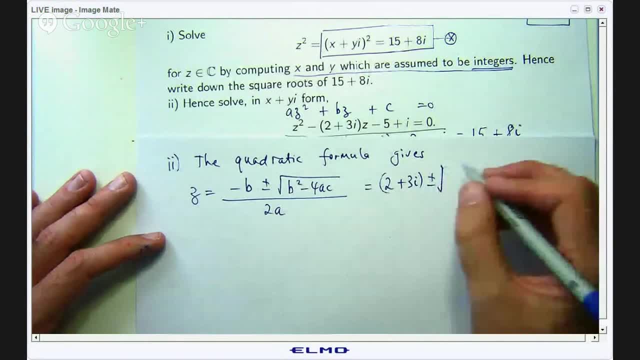 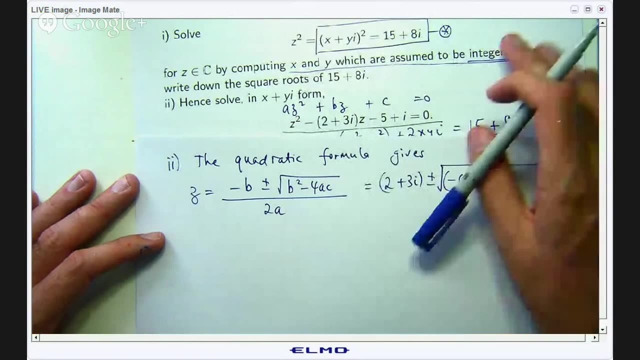 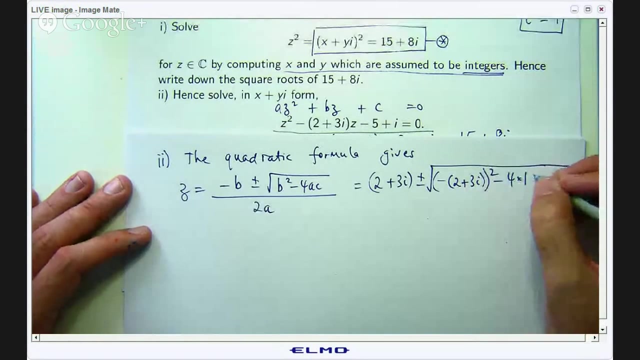 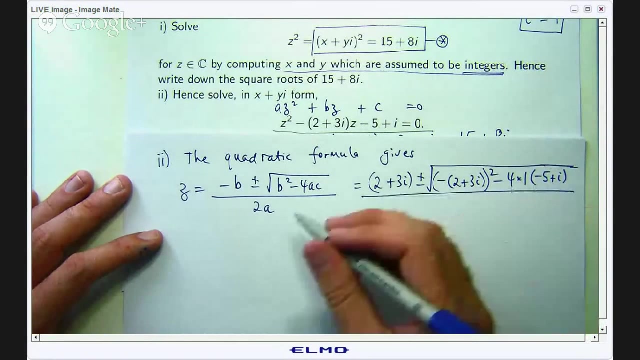 Okay, b squared, that is going to be this, That is going to be this, So that is going to be this. Okay, So that is going to be this. Okay, Minus 4 times that, times a and a is 1, okay, I just squeezed it in. all over 2a, a is 1.. 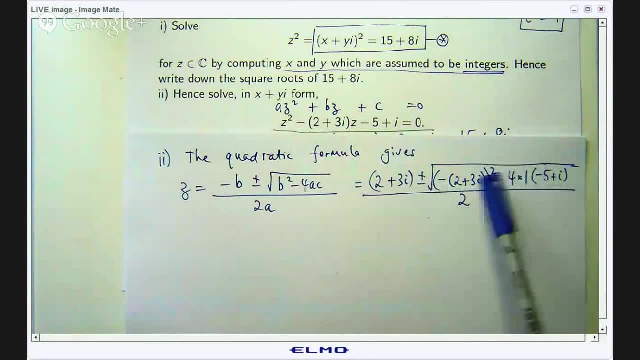 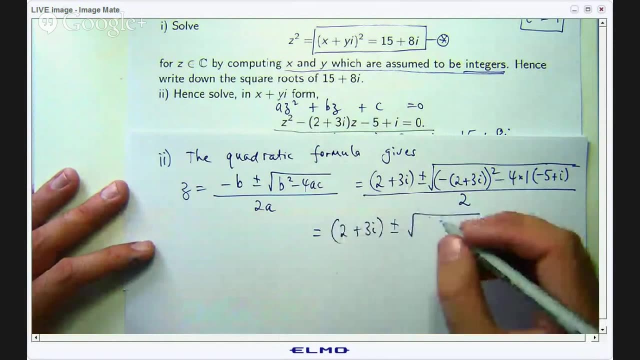 Okay now, this is a bit of a mess here, but if you expand this out, you will get inside that square root sign: 15 plus 8i. now I am not going to put the details in. if you want to fill them in, you can yourself. 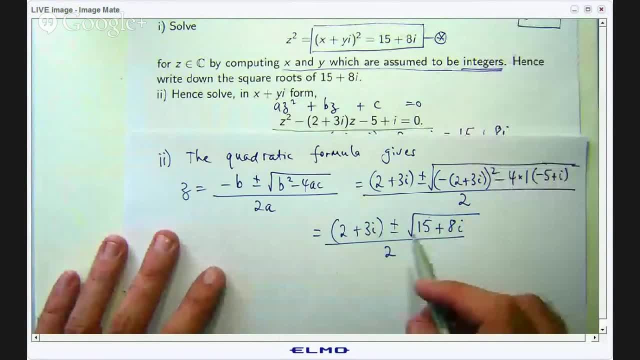 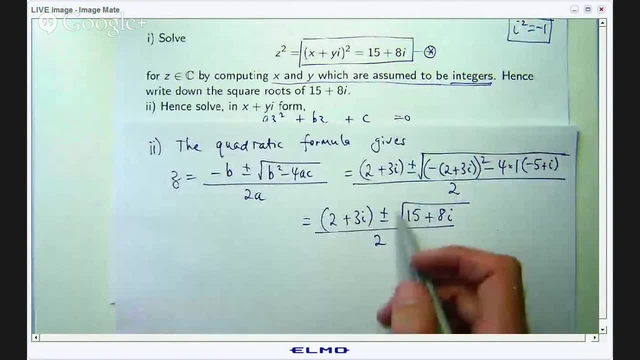 Okay, so now, because we have computed the square roots of 15 plus 8i in part i, I can actually write an expression down for this. okay, We got them to be this and this: I have already got the plus or minus there, so I am going. 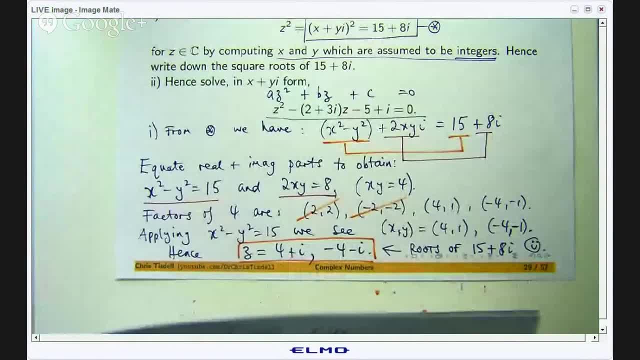 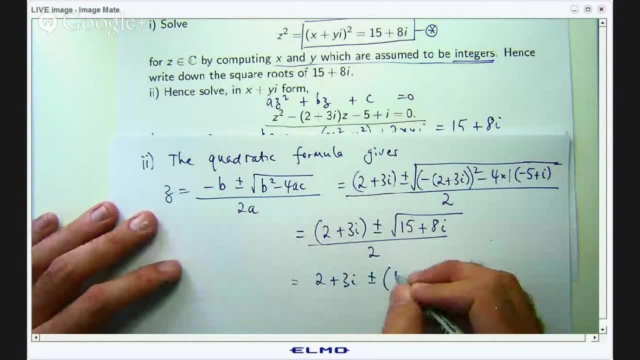 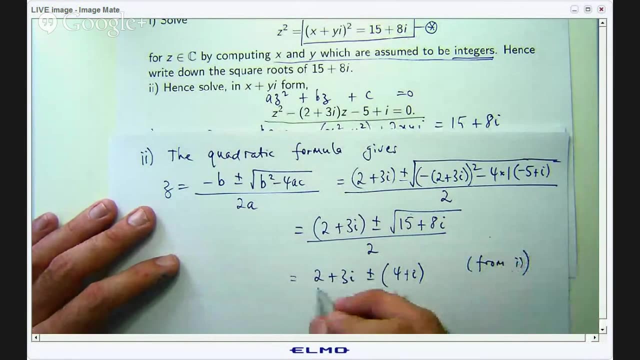 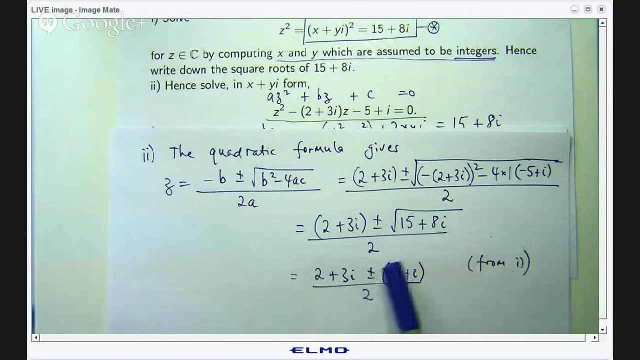 to replace the square root with just say 4 plus i. So that is from part i or part 1, so now all we have to do is simplify. okay, So if I use the plus sign, I am going to get 2 plus 4.. 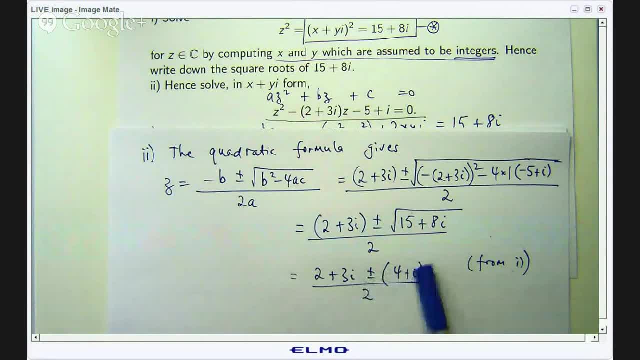 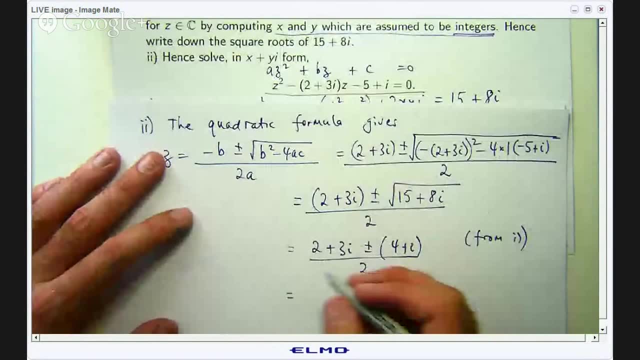 Which is 6 plus 3i plus i. so I am going to get 6 plus 4i all over 2.. So if I divide the 2 in, I will get 3 plus 2i, and if I do the negative sign, 2 minus 4. 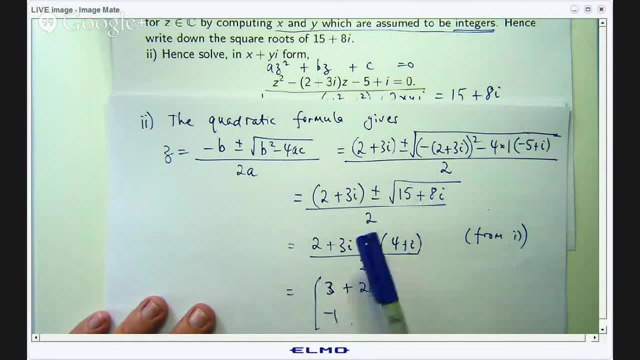 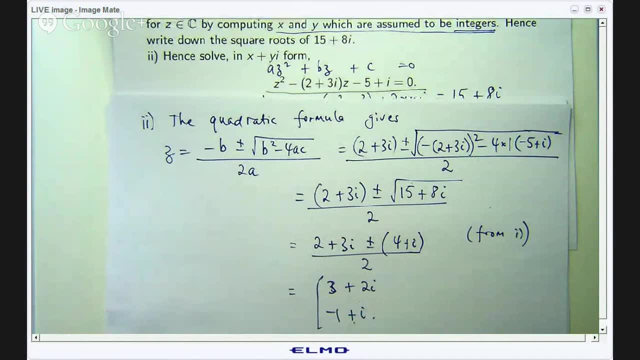 that will be negative. 2 all over 2, that will be negative 1, and the 3i minus i, that is 2i all over 2, that will be plus i. okay, So the solutions to that quadratic equation are given Okay.